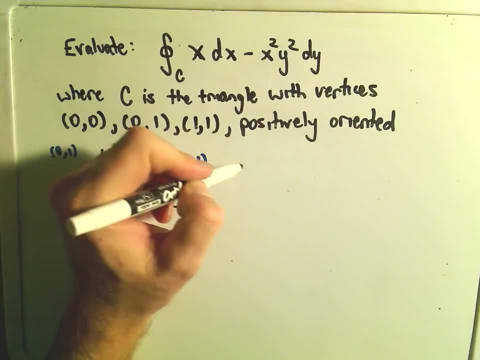 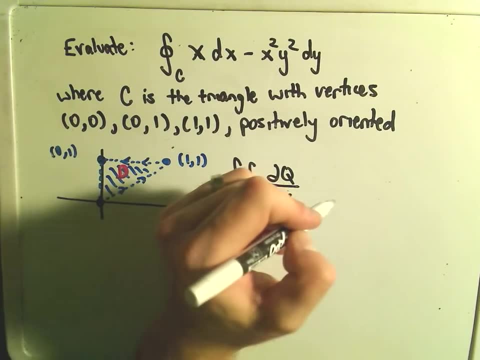 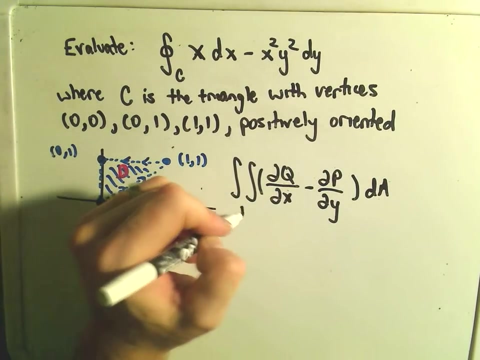 And it says all that we do is we just go from our line integral to a double integral. It says we take the partial of Q with respect to X, Minus the partial of P with respect to Y over our region, And again, just the way we had things labeled a second ago. 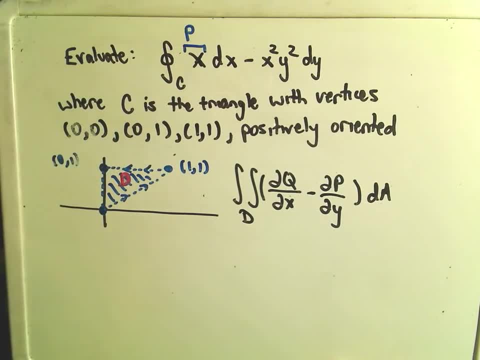 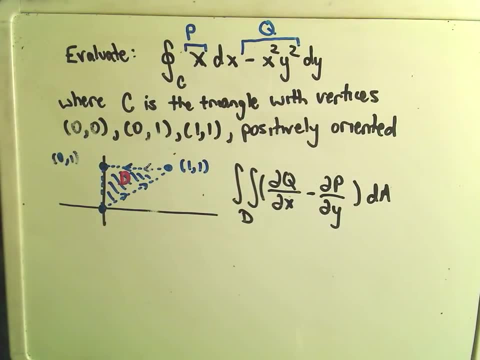 Whatever's in front of the DX, that's our P function, And whatever's in front of the DY, that's going to be our Q function. So make sure that you include the sign there. Okay, so we'll figure out the limits of integration here in just a second. 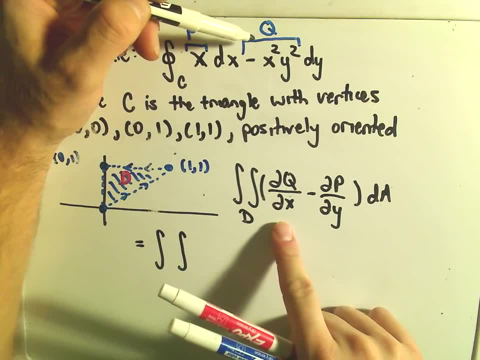 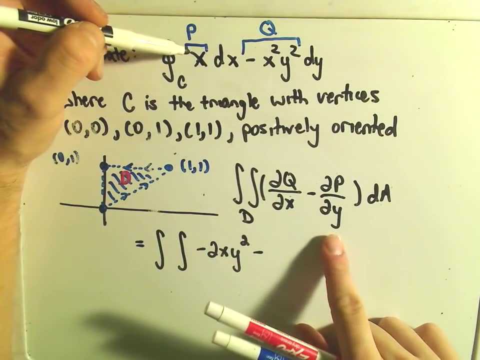 But it says: if we take the partial of Q with respect to X, to me it looks like we're going to get negative 2X, Y squared Minus. then we take the partial of P with respect to Y, But there we treat X like a constant. 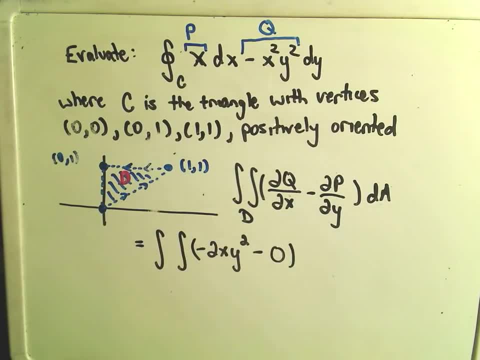 So that actually just becomes 0.. I think I'm going to integrate this one with respect to Y first And then with respect to X. So remember, if we integrate with respect to Y, our lower limit of integration is whatever the bottom curve is. 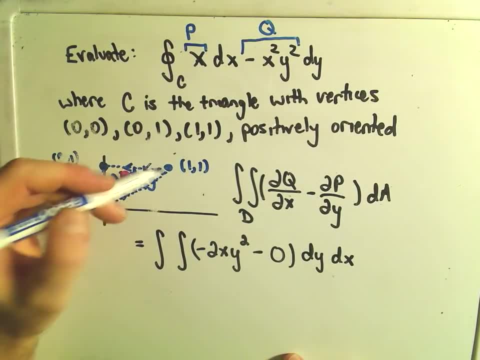 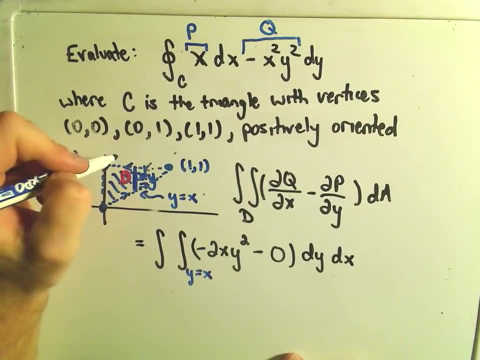 And since it's just a line that goes from 0 to 0, 0 to 1, 1.. This is simply going to be the curve. Y equals X, So we'll be integrating from Y equals X. The top part is the horizontal line. 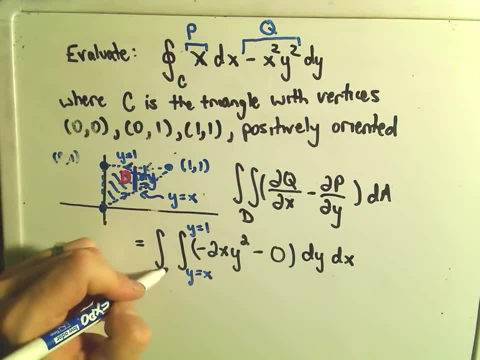 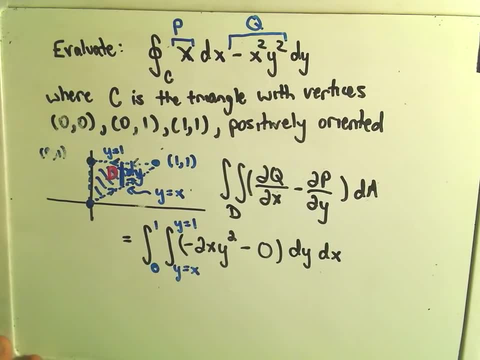 Y equals 1.. Then our X values just range from 0 to 1.. So now we've used Green's theorem to set up the double integral that we have to calculate. Um, So again we've turned a line integral into just a double integral. 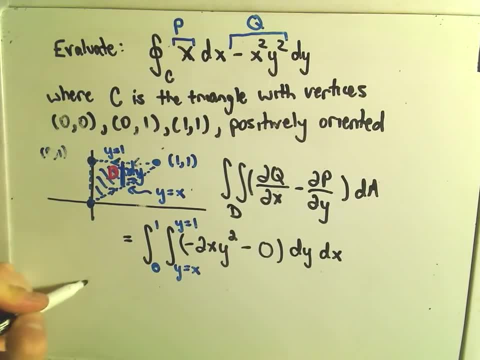 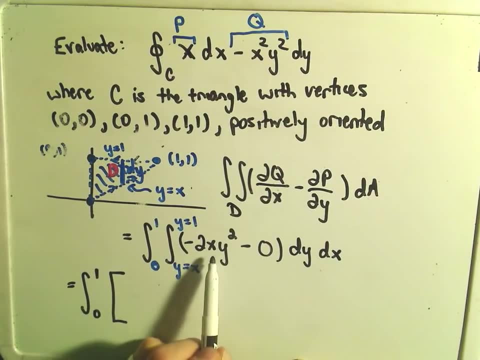 So hopefully this one won't be too bad to compute, So let's just go ahead and grind it out here. We'll have to integrate from 0 to 1.. You've got to integrate negative 2X squared- excuse me, negative 2X Y squared. with respect, 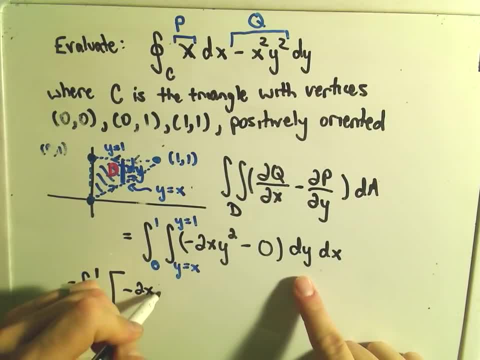 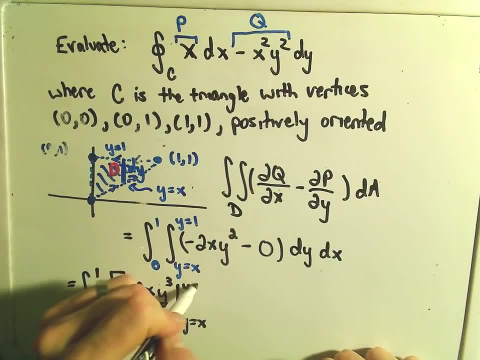 to Y. So we treat the negative 2X like a constant. When we integrate we'll get Y cubed over 3. We'll have to evaluate that from Y equals X to Y equals 1. And then integrate all that with respect to X. 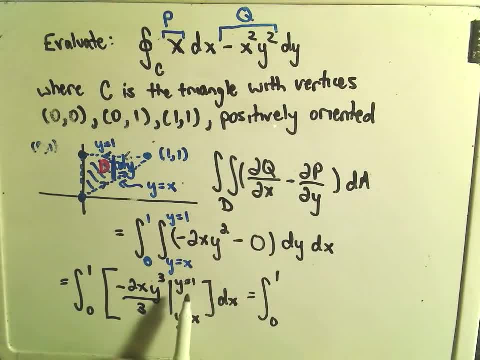 So again, not too bad, just a little tedious. If we plug in the upper limit, Y equals 1, we'll get 1 cubed, which is 1.. So we'll get negative 2X over 3.. We'll subtract away the lower limit, which will give us a positive. 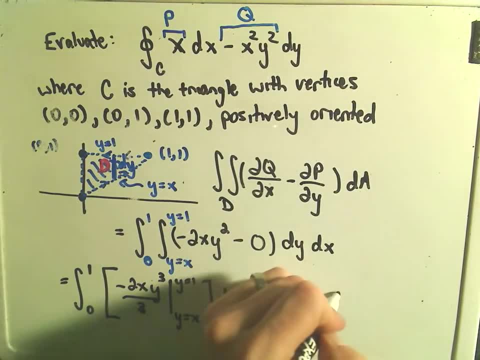 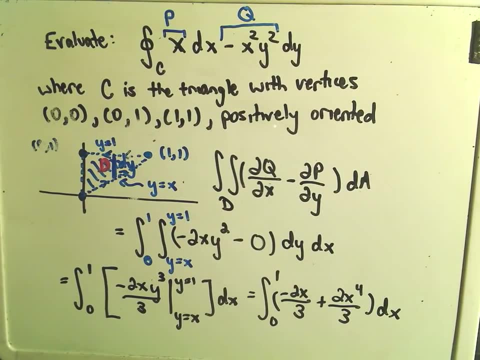 When we plug in X, it looks like we'll get 2X to the fourth again over 3.. And that's what we have to integrate now with respect to X. So pretty close. Let me give myself some more room here, real quick. 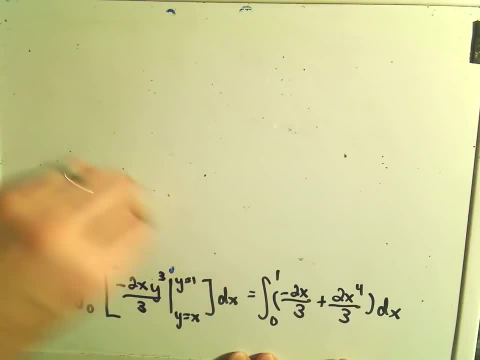 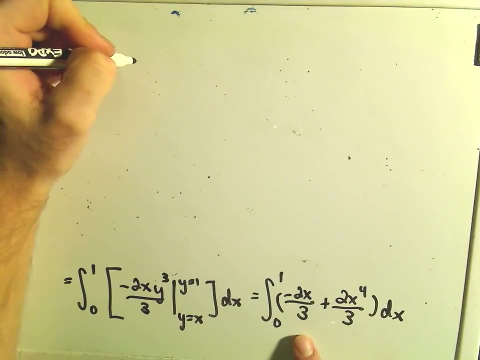 This is about as easy as an integral is going to happen in a Calc 3 class. I think So, if we integrate this last integral with respect to X. so let me just go ahead and do it in one fell swoop, I guess. let's see. so the negative 2 thirds looks like we'll get, so I always just do. 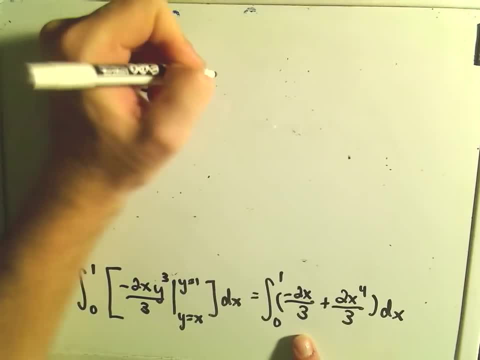 it So negative 2 thirds. we'll get X squared over 2 plus 2 thirds, And then we'll get Y squared over 2 plus 2 thirds, And then we'll get Y squared over 2 plus 2 thirds. 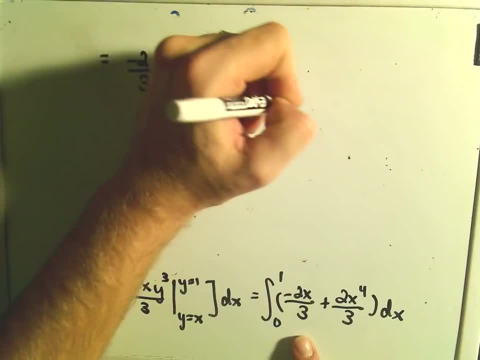 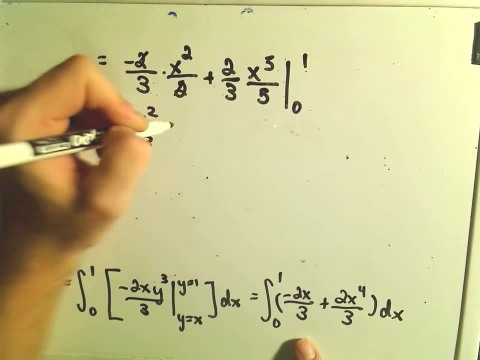 And then we'll get Y squared over 2 plus 2 thirds X to the fifth over 5.. We have to evaluate that from zero to 1.. So, okay, the 2's cancel. So that's negative X squared over 3.. 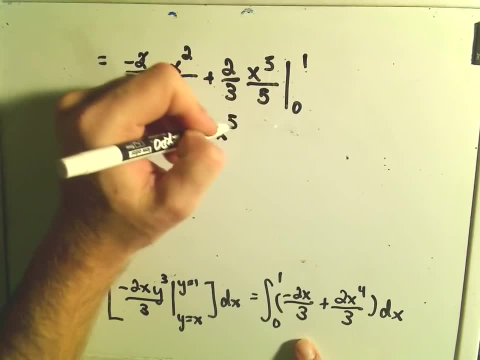 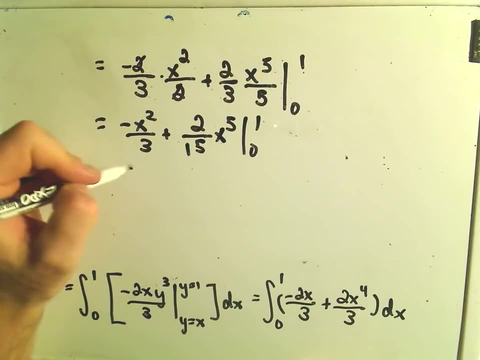 It looks like 2 over 15, X to the fifth, from zero to 1.. So if we plug in our upper limit, 1, we have to square the 1 first. So we'll get 1 squared. we'll get negative 1 third plus 2 over 15, 1 to the fifth being. 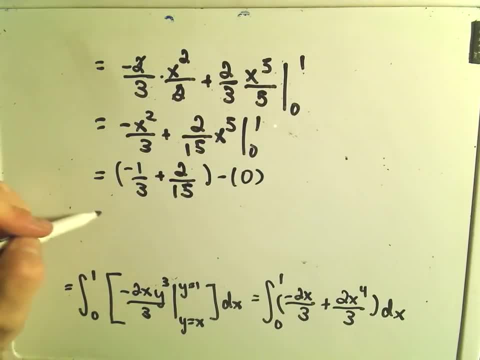 1. And then our lower limit. we're just going to get a bunch of zeroes. So let's see, if we get common denominators top and bottom by 5, we'd have negative 5 plus 2, which would be negative 3 over 15, or the value negative one-fifth. 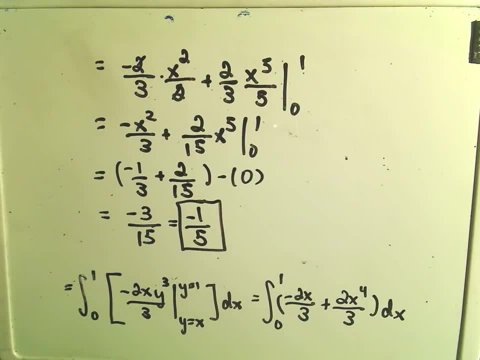 So again, basic idea it says in some cases you can turn line integrals into double integrals. is all it says, And a lot of times evaluating a double integral might be a little bit easier than evaluating a line integral. That way you don't have to figure out usually a good parametric representation. 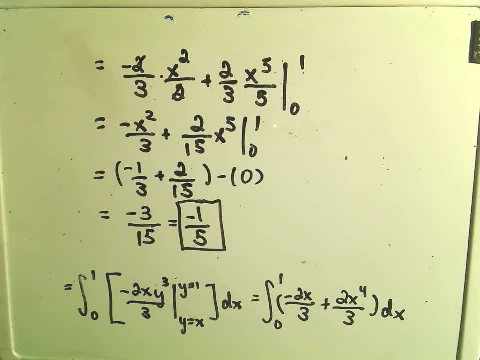 I think they're just a little bit more straightforward. So, alright, I hope this example helps, makes some sense. I'm going to do definitely a more complicated one, perhaps, where you have to use polar coordinates to integrate, but that'll be in another video.